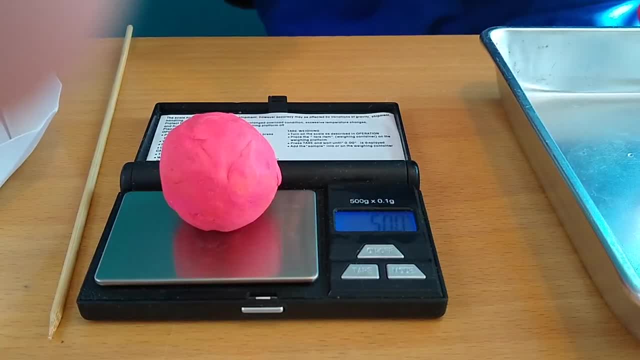 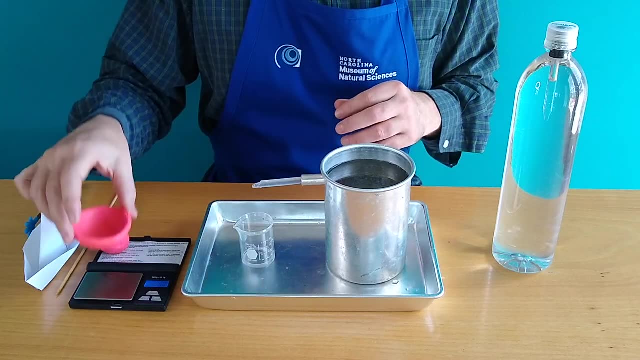 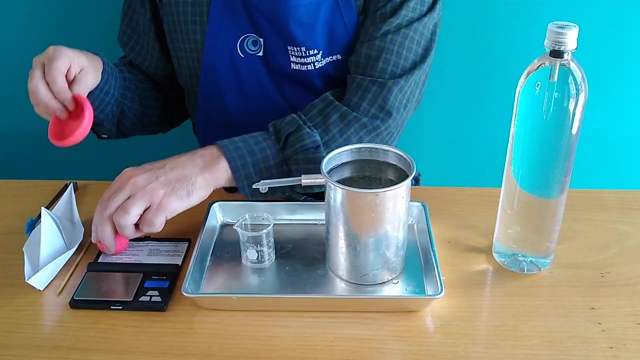 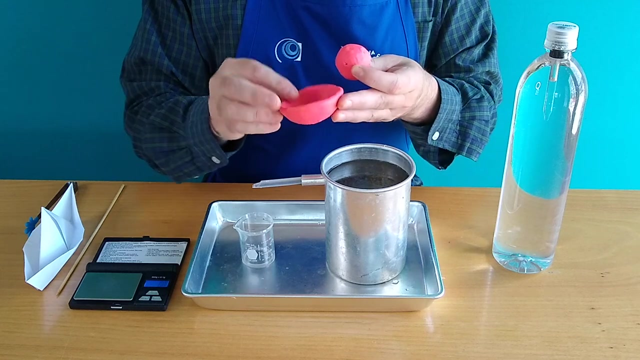 It weighs. let's see here about 50 grams. Now let's weigh the clay boat and see how much it weighs For our experiment. I hope it's close And it too weighs 50 grams. So both objects are made out of clay, Both weigh 50 grams, but only one of these two is actually going to float, And you. 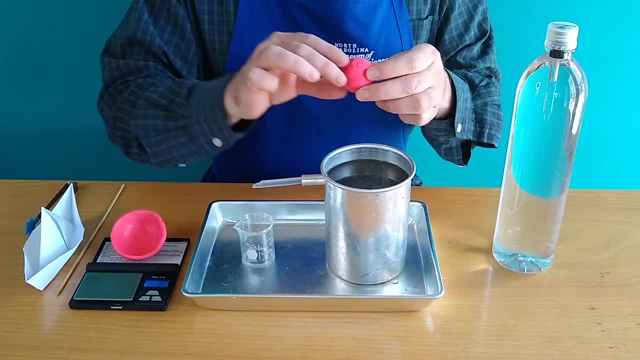 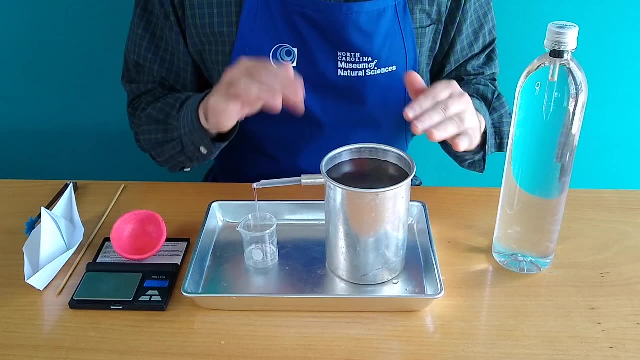 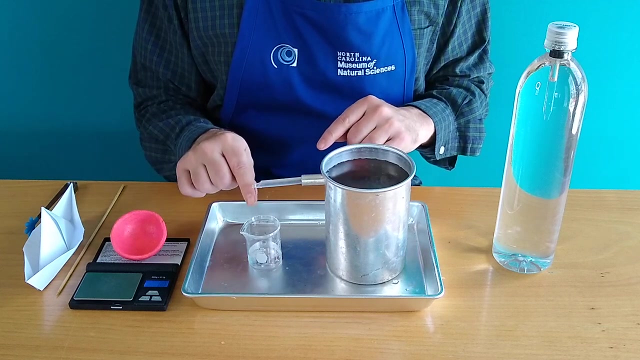 probably guessed which one's going to float or sink. Let's start with the clay ball. Let's place it on this displacement tank And, not surprisingly, it sank like a rock And a bunch of water is coming out on this end. How much water comes out? Well, if we wait long enough for all. 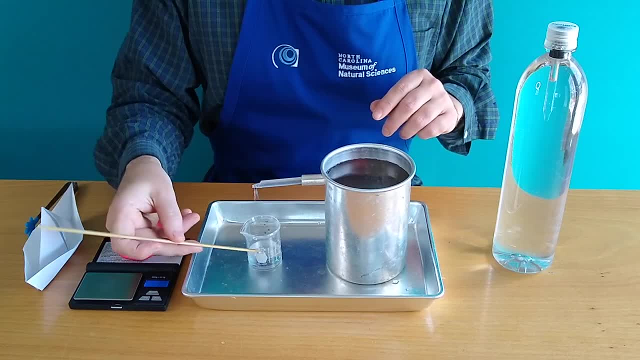 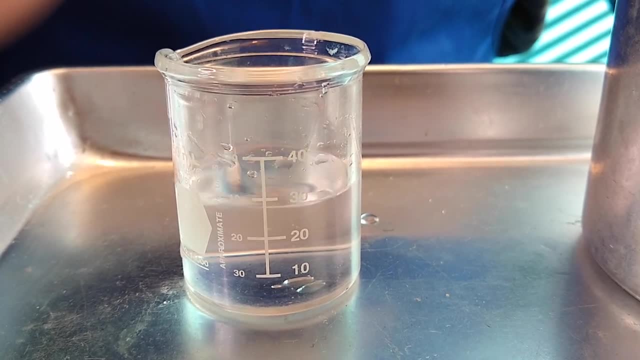 the water to drip out. that would drip out. it would come out to about 30 milliliters. on our graduated beaker That is equal to the volume of this clay ball. That is how much space it takes up. But what we're really interested in today is not something sinking, but more about why is it? 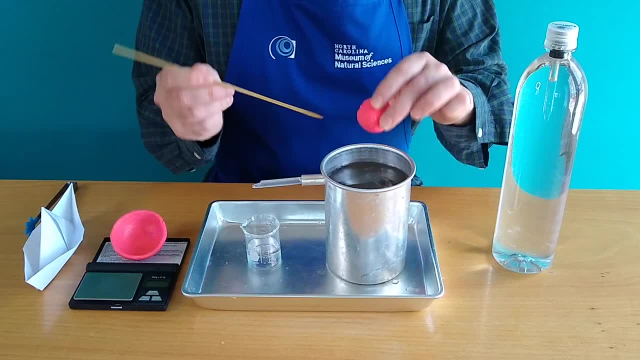 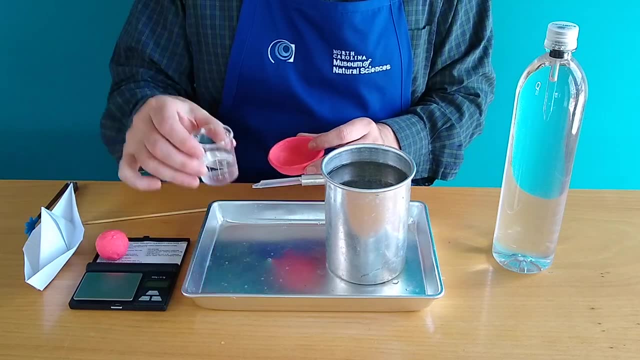 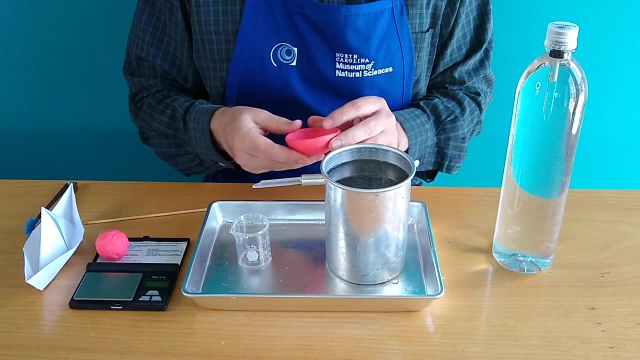 something floating. So let me fish this ball out of the water, And this time let's float the clay boat. Now, to do this precisely, we have to pour this water back in, So we're back at zero, Because really you can look at this like a digital or not digital scale, but a water scale. I need some. 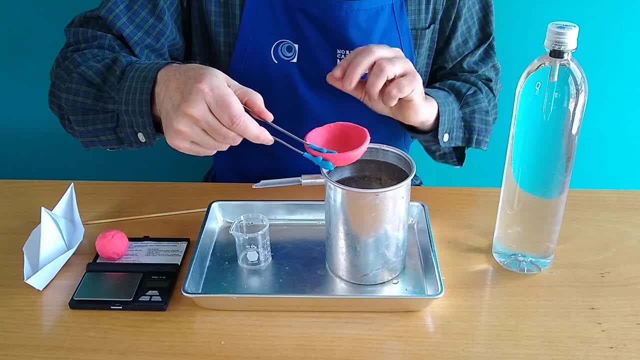 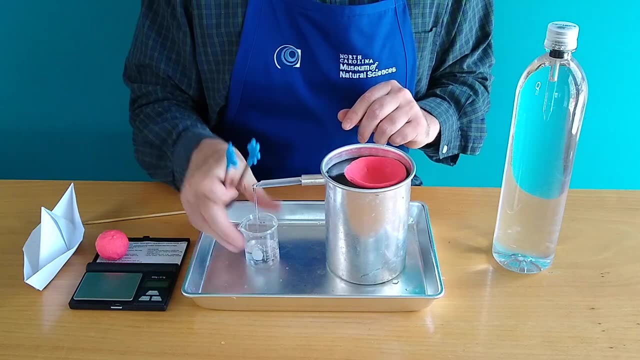 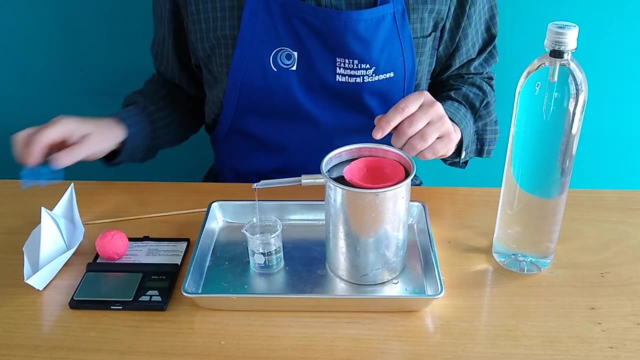 helping hands to help place this boat. I've got my little hands here. Let's carefully lay this on top of the water. It's floating and it's pushing out a volume of water. Now, this time, the amount of water that comes out on this side is not going to be 30 milliliters. It should be 50 milliliters at least. 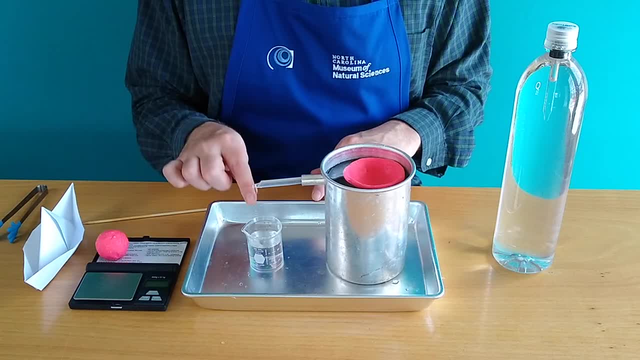 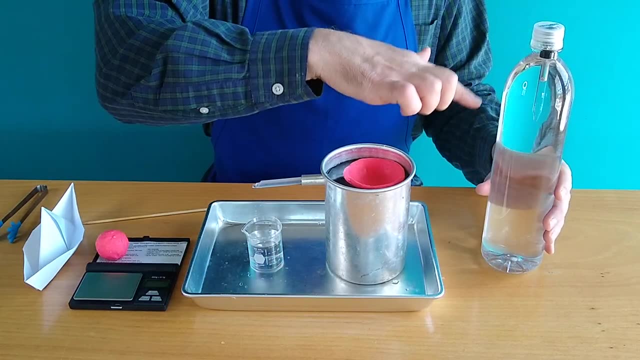 if Archimedes was correct. Now, while we wait for this to drip and get up to that point, let's take a look at the Cartesian diver that we saw earlier. Why was this thing sinking and floating in the first place? Why was it magically following my finger? Turns out it has nothing to do with my. 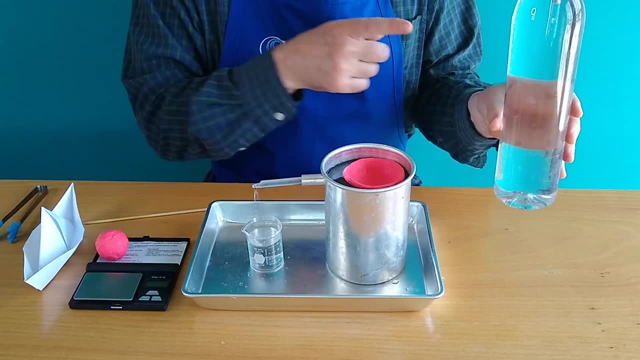 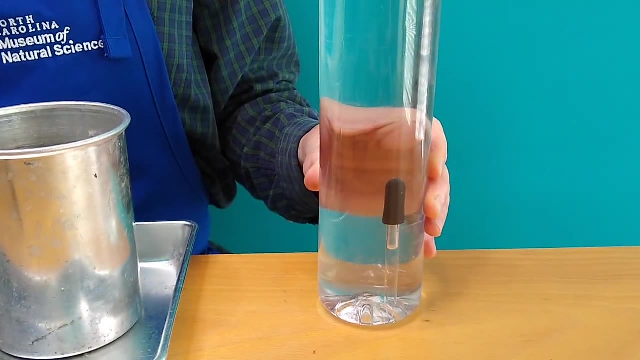 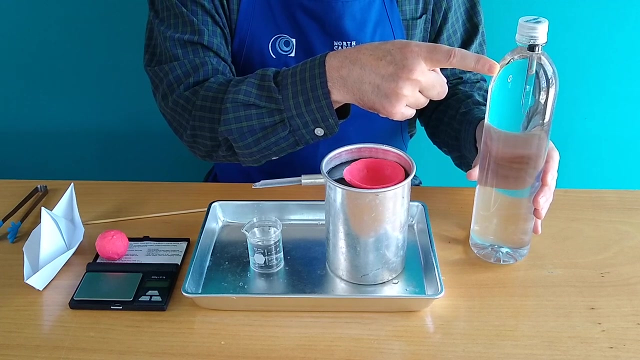 following my finger. what I was doing was I was just changing the density of this eyedropper by squeezing the bottle and letting go. squeezing the bottle and letting go, it turns out if you look closely up here at the eyedropper, you'll see that there's actually an air bubble. that air bubble is pushing out about 4.